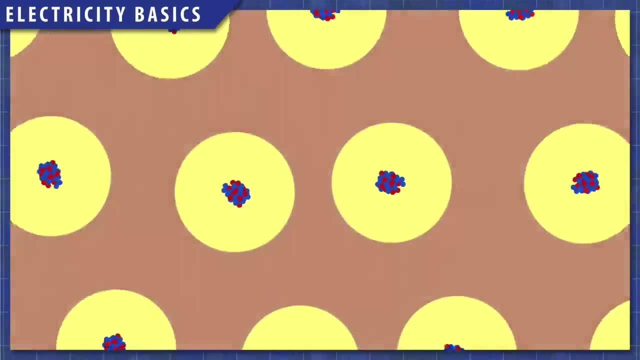 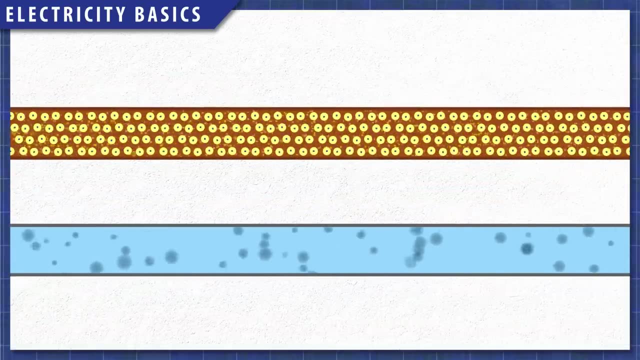 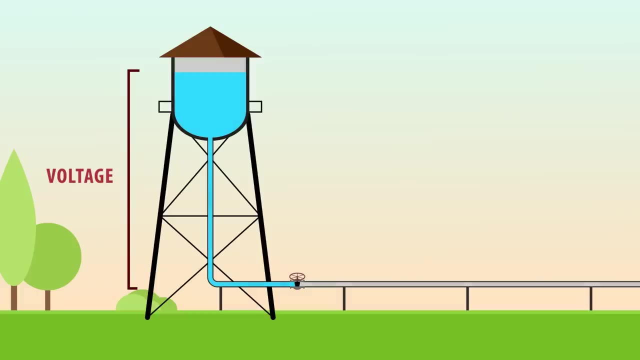 Electricity is the movement of electrons from one atom to another. The flow of electrons through a wire is somewhat similar to the flow of water inside a pipe. Voltage or potential difference is the pressure from the power source that pushes the electrons through the wires. 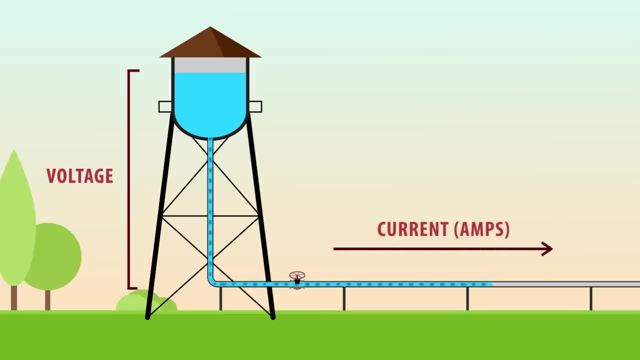 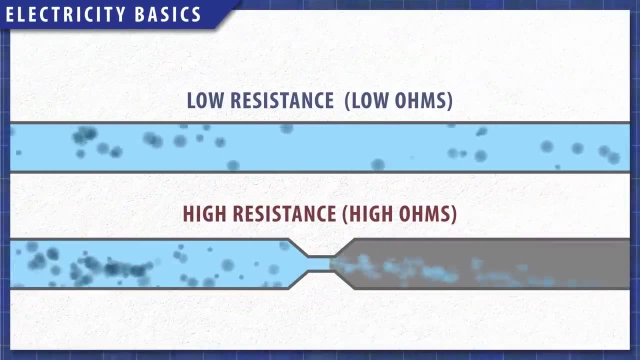 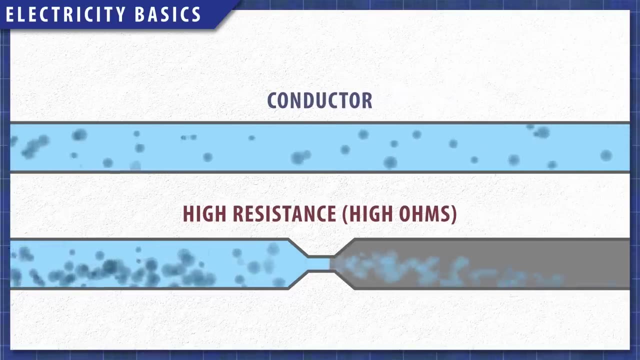 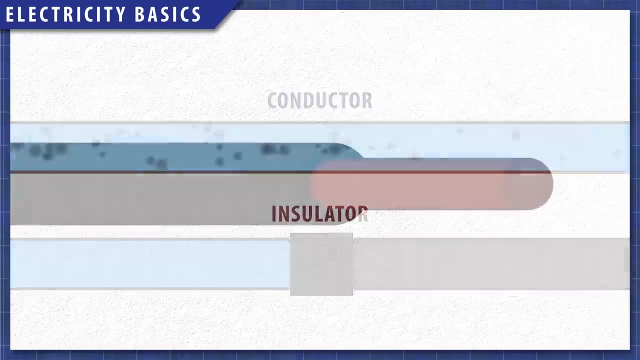 Current or amperage is the flow of electrons within a circuit. Resistance measured in ohms is the amount that a material will resist the flow of electrons. Conductors have low resistance, allowing electrons to move easily through them. Insulators have an extremely high resistance to the flow of electrons. 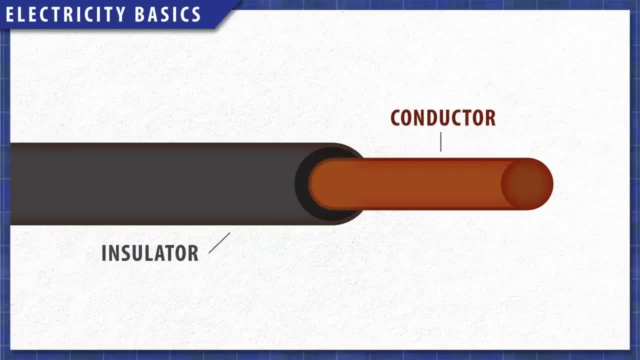 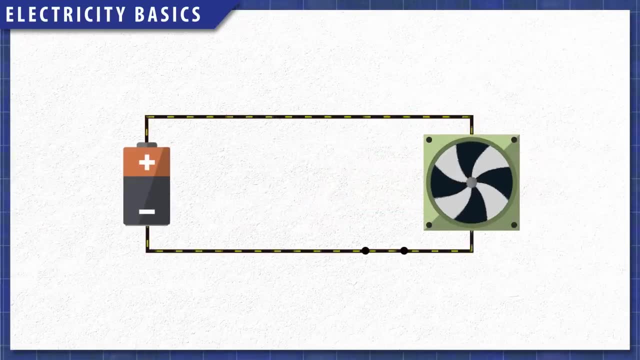 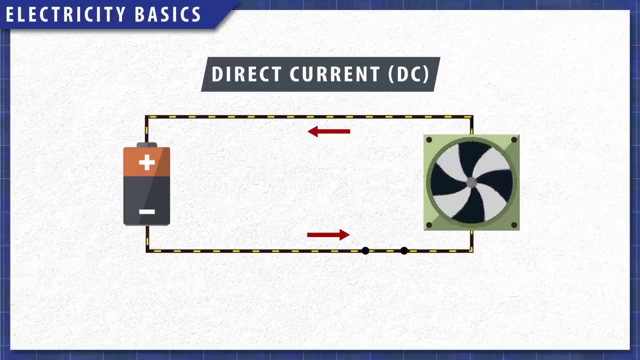 For example, copper wire is insulated by a plastic sheath. If we connect these wires together to a power source, we get a complete electrical circuit. Batteries provide direct current or DC power, as the current always flows in a single direction. 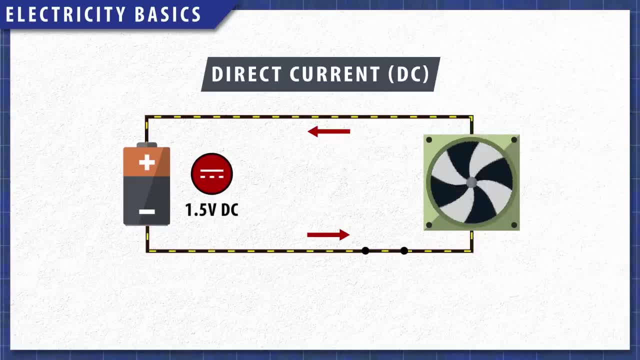 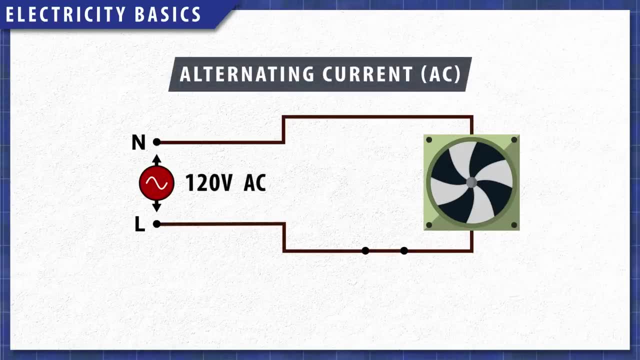 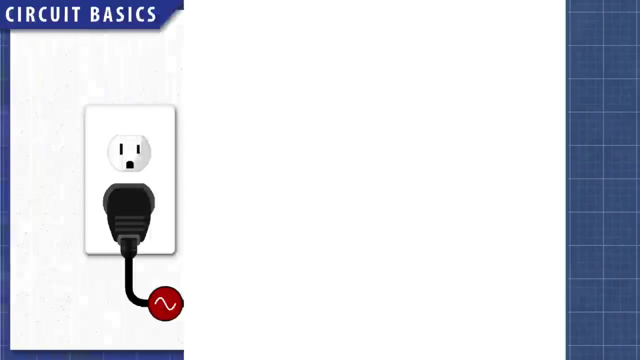 This is represented by a dash line on the multimeter. Your home is run off 120 volts alternating current or AC power. The direction that the current flows is changing 60 times a second or at 60 hertz. This is represented by the sine wave. 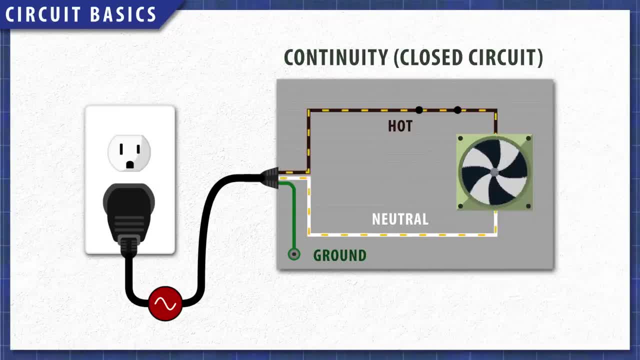 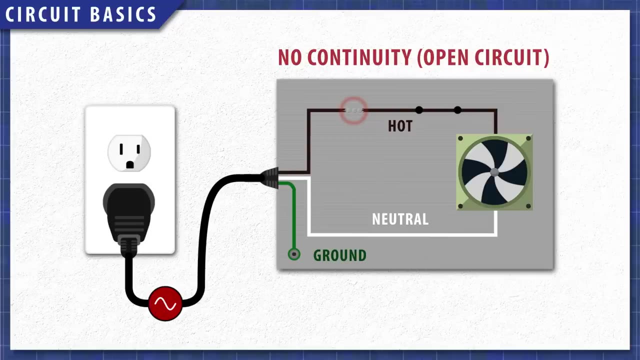 In either case, the electrons always need a continuous path to return to the source. This is continuity or a closed circuit. If we disrupt this path with rubber, plastic or by air in the case of a broken wire- the electrons will not flow, as there is no continuity. 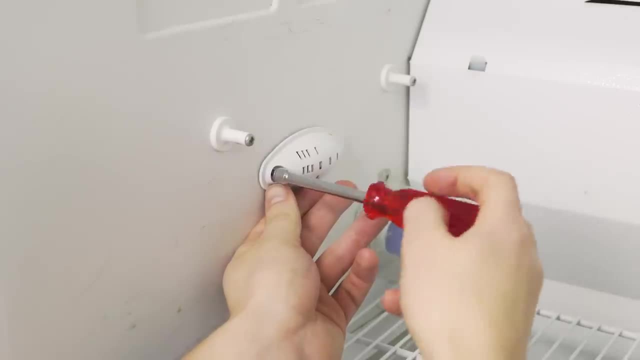 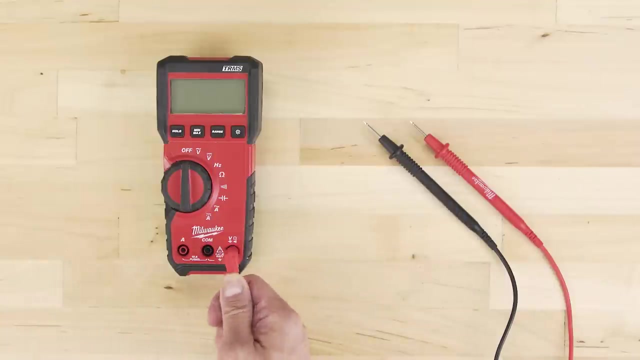 This is an open circuit. In many cases the lack of continuity in a single component will prevent an appliance from working properly. To set up the multimeter plug the meter leads into the terminals. Usually they are color coded: red for positive and black for neutral or common. 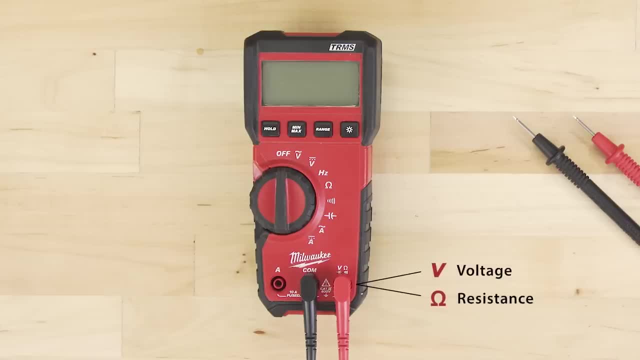 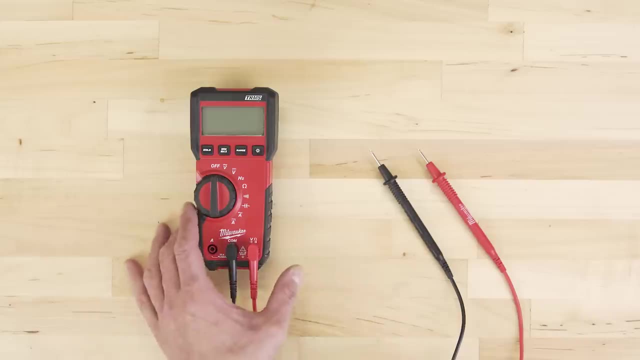 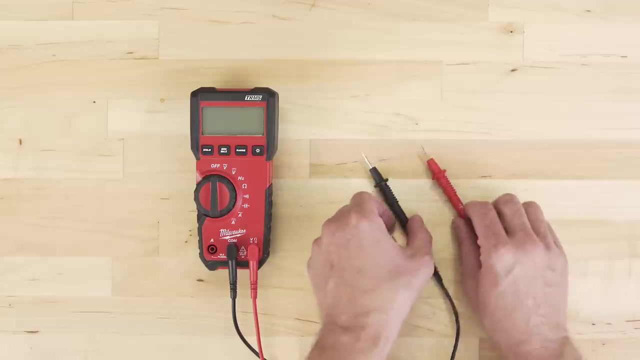 Some meters will have two positive terminals. One terminal is for voltage and resistance and the other is for measuring amperage. Always inspect the multimeter before use. Never use a multimeter that has a damaged case or test leads with nicked or damaged insulation. 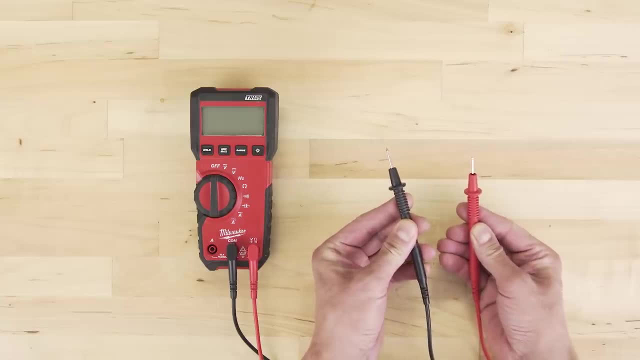 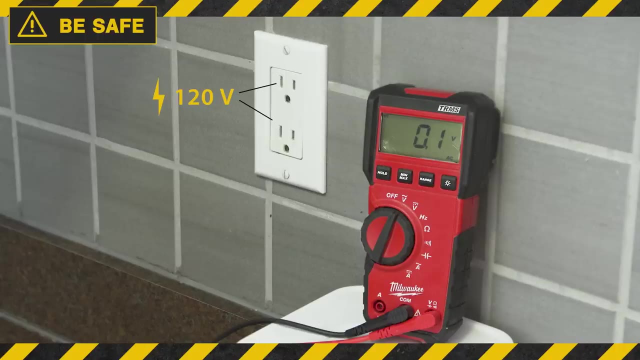 To be safe, always hold the multimeter from the insulated handles. Even 120 volts in your home can be deadly, so use caution before testing any live voltage. If you're unsure at any point, then it's best to contact a professional. 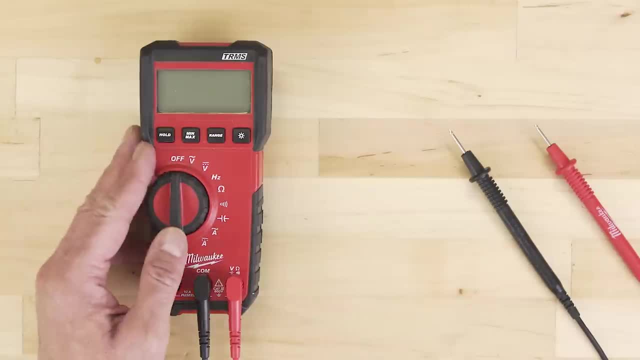 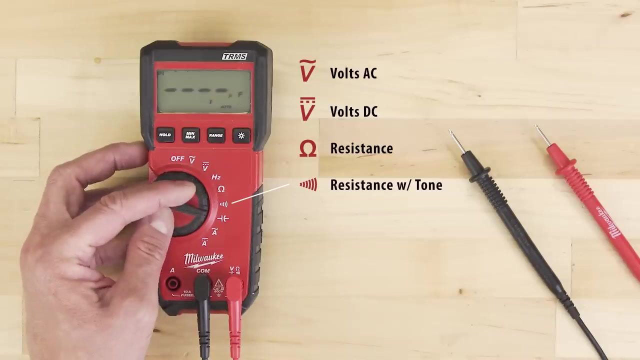 Your model might look a little different, but all multimeters have the same common controls: Volts AC, Volts DC, Resistance in ohms And resistance with tone, Which will beep when there's continuity As well. you can test for capacitance. 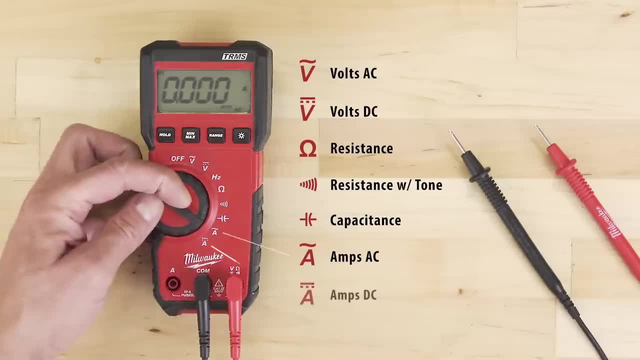 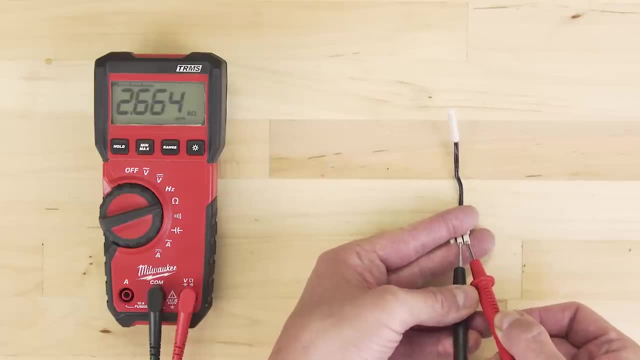 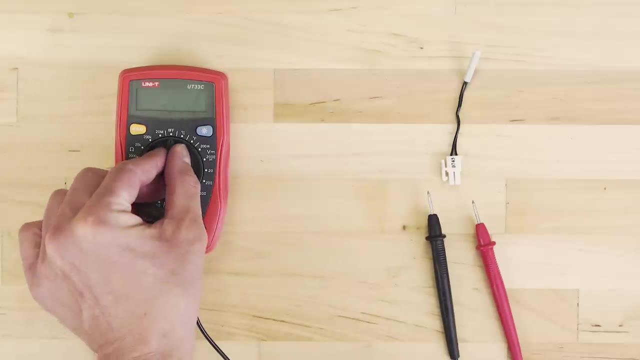 Amps AC And amps DC. Some multimeters are auto-ranging and will automatically adjust the units displayed In other models. you'll have to set the multimeter to the most accurate range, For example, if we test continuity at the 20kts. 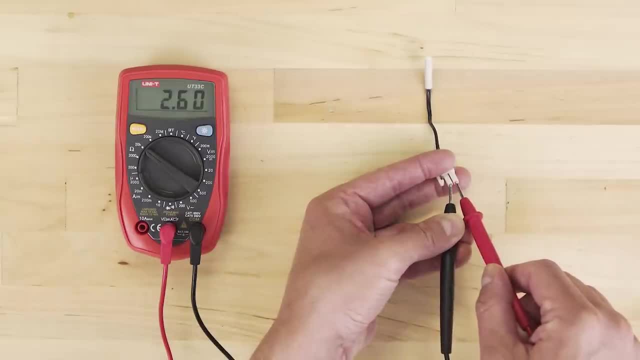 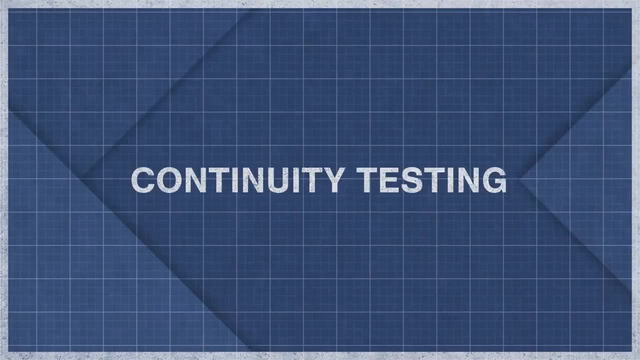 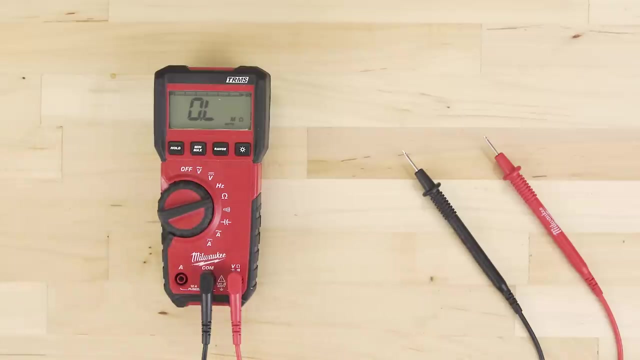 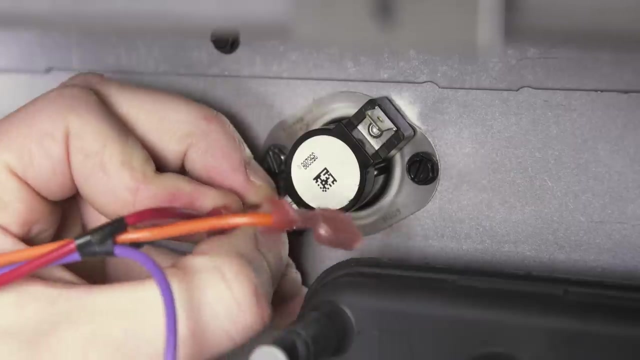 and we get a reading of 2.6, then the resistance is 2600 ohms. To test a component for continuity, first set the multimeter to the ohms or resistance with tone setting, Safely disconnect the power and remove the wires or connectors. 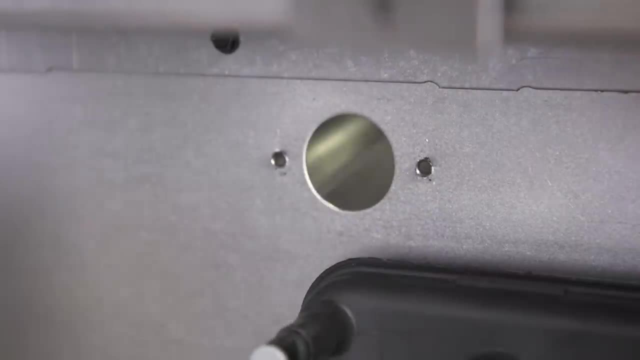 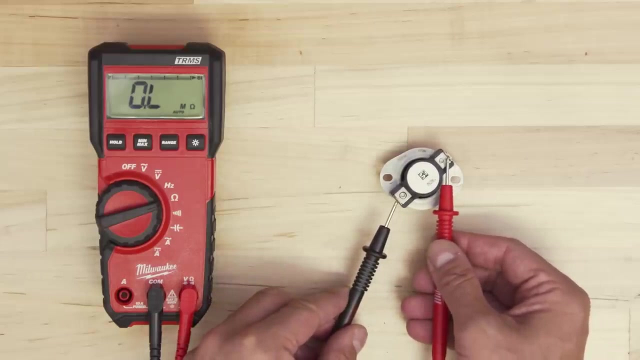 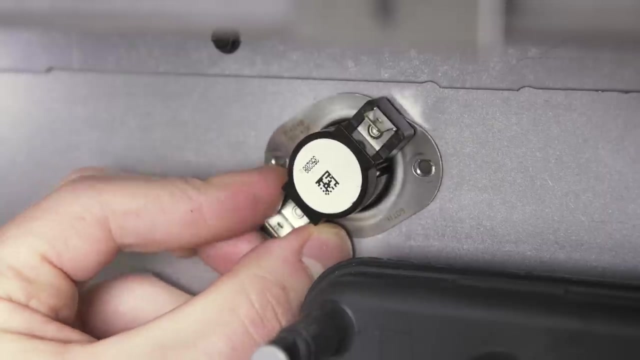 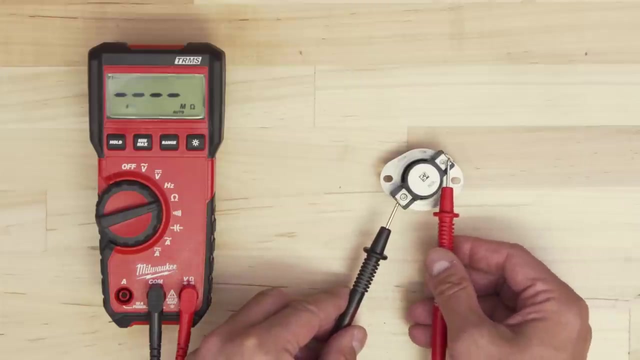 Now remove the component or isolate it. Next, touch each probe to each component terminal. If there is no continuity, then the multimeter will display OL or open loop. This means the component will need to be replaced. If there is continuity, you'll get a reading above 0 ohms. 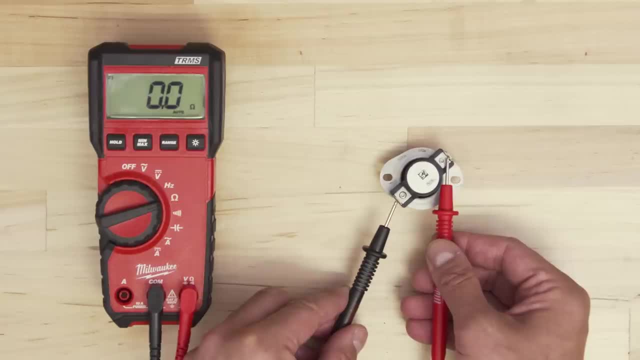 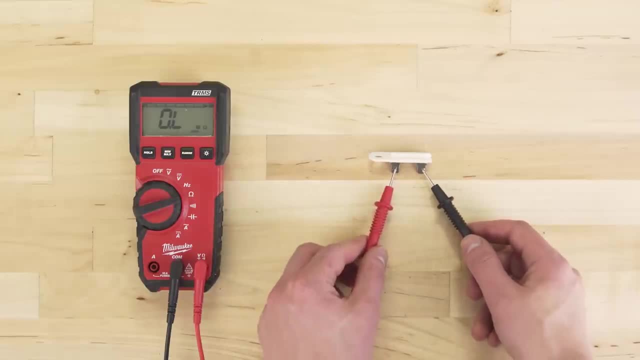 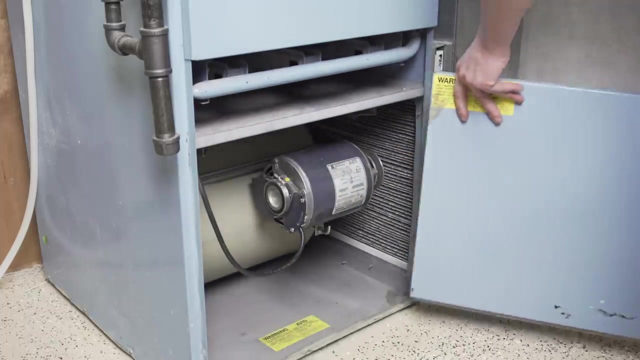 provide an unrestricted path for the electricity to pass through. These will typically have a resistance reading between 0 and 1 ohms. Load components include heating elements, solenoids, motors or any component that consumes power. They will need a specific resistance value to function correctly. 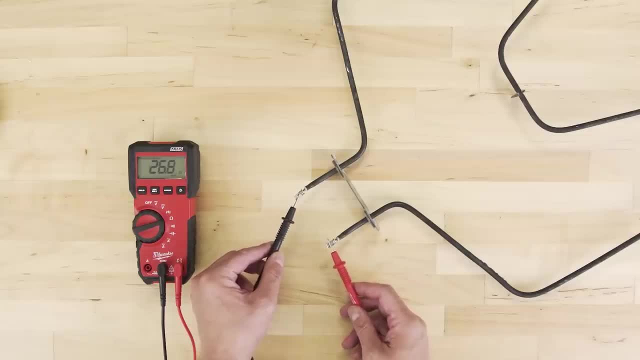 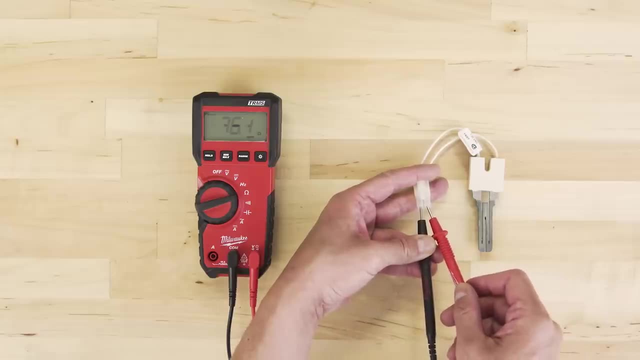 For example, oven bake elements commonly have a resistance of 20 to 40 ohms, whereas hot surface igniters can range from 30 to 200 ohms. This is different for each component and will vary between models. If you want to learn more about the various components and appliances, 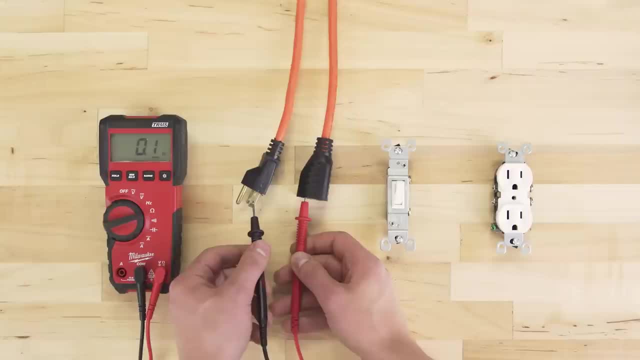 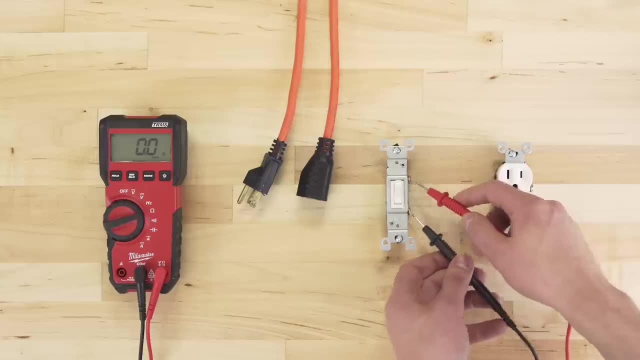 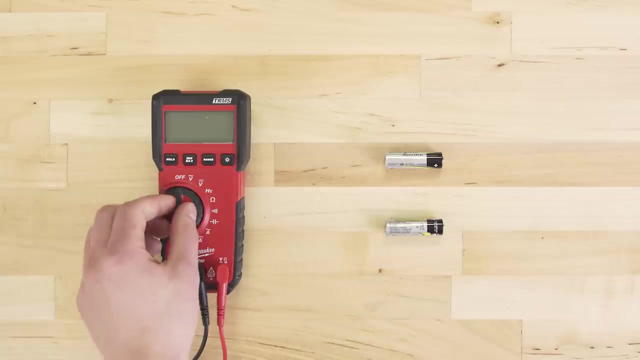 then watch the video linked below As well. continuity tests can be useful when trouble occurs. For example, you may have trouble shooting other electrical items in your home. This includes extension cords, light switches and receptacles. The volts DC setting can be used to test batteries and other small electronics. 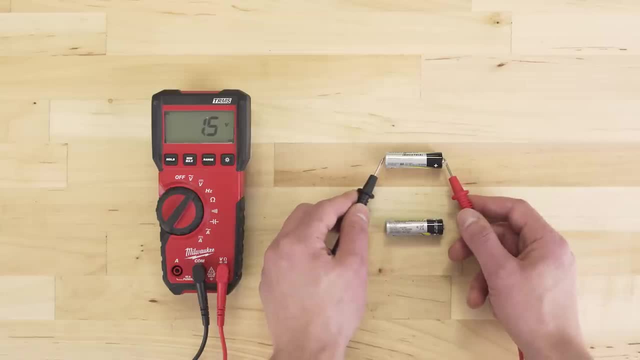 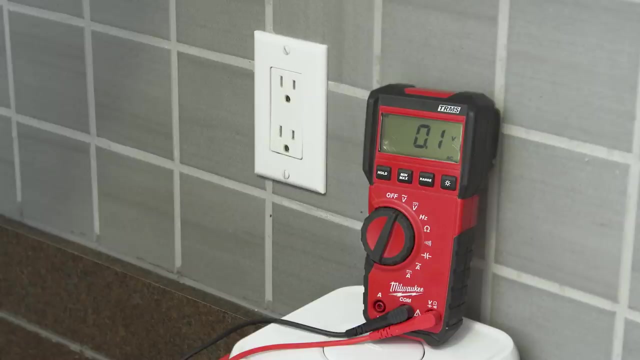 For example, a fully charged AA battery will be close to 1.5 volts, whereas a weak battery will be more likely to overcharge, much lower at 1.2, and should be replaced. By setting the multimeter to volts AC you can test to see if a receptacle has power. 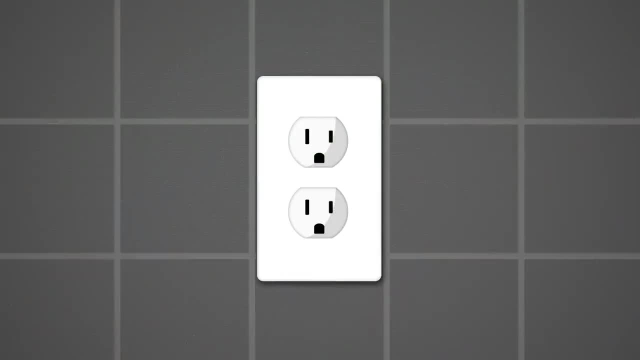 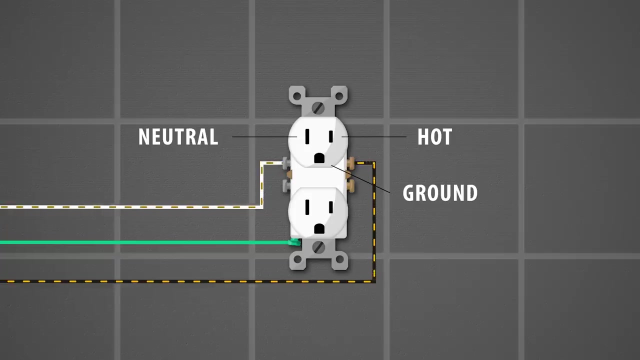 and is wired correctly. The small plug is the hot wire that is providing the power. The larger plug is the neutral wire, which returns to the power source. The rounded plug is the ground wire If at any point a hot wire touches the metal casing. 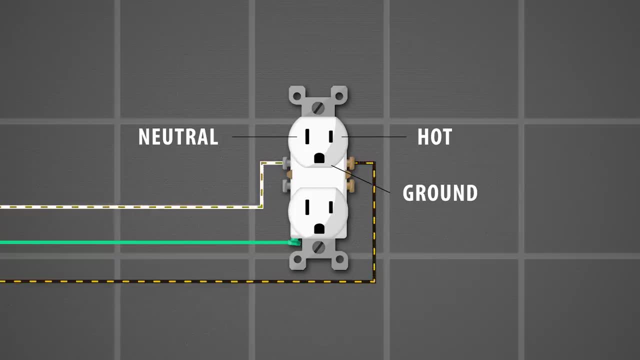 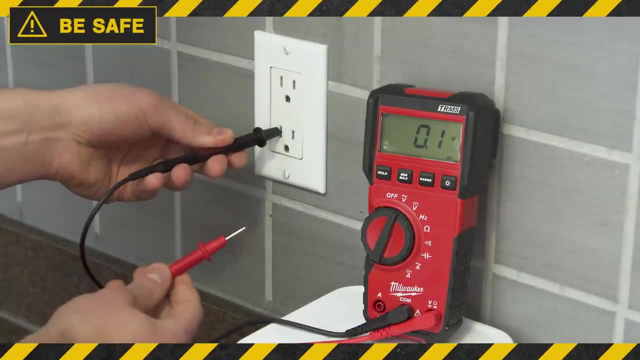 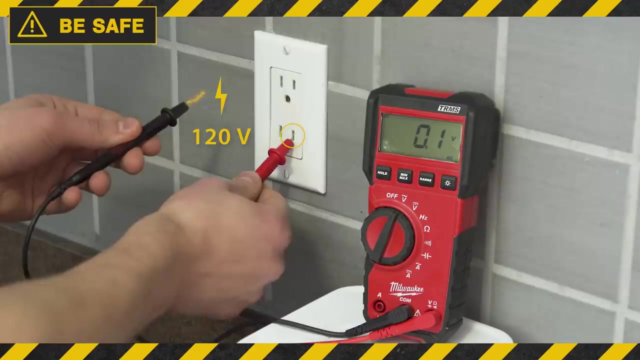 the ground wire provides a safe return path back to the source. When testing live voltage, it's essential to use caution. Always start with the neutral wire first before connecting to the hot. If you connect to the hot side first, the other multimeter probe now becomes energized. 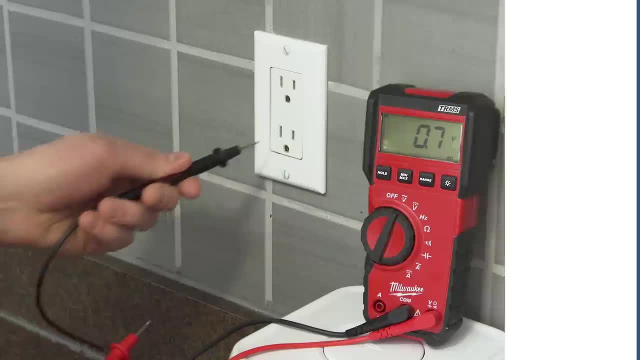 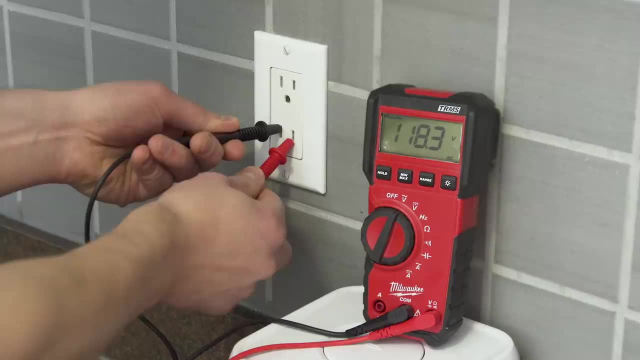 which increases the risk of a shock. Testing from neutral to hot will show approximately 110 to 120 volts. Testing from ground to hot will also show around 120.. This will verify if the ground wire has a complete path back to the breaker panel.